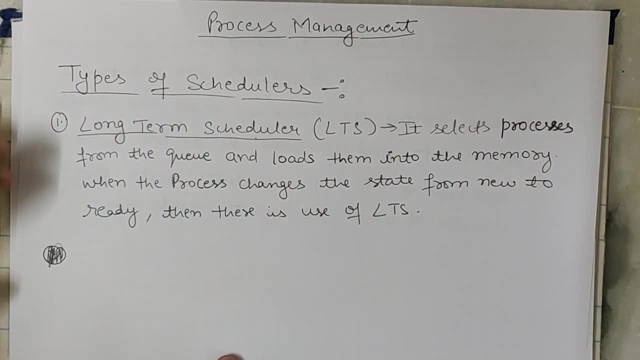 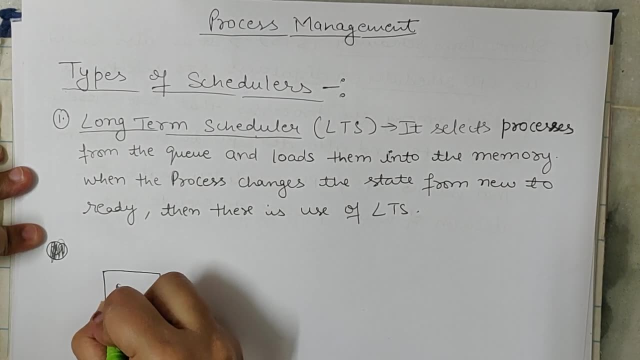 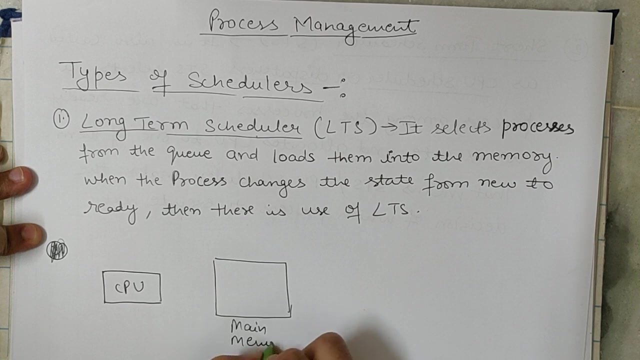 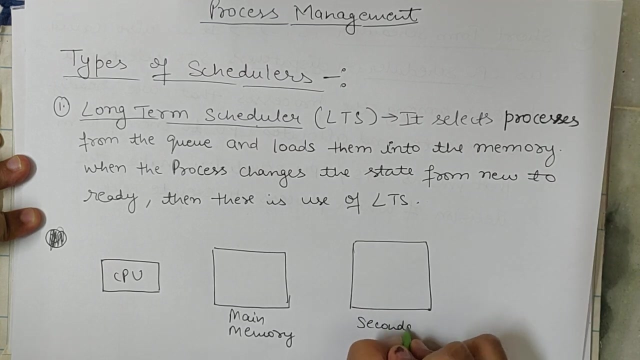 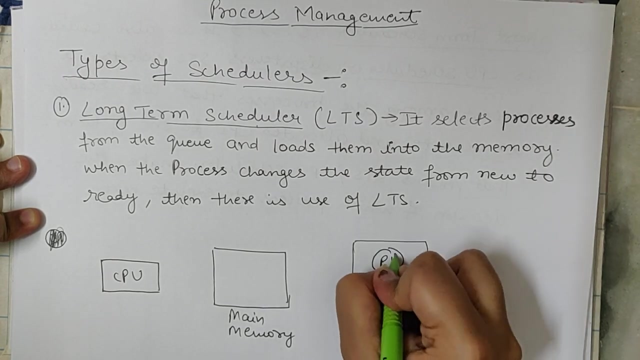 the first one is long term scheduler. let's explain this. let's i will explain it with the help of an example. this is cpu, this is a main memory- okay, main memory. and this is secondary memory- okay, so this is my program. p1 lts ki job, kya hai, it moves program if i want to execute a. 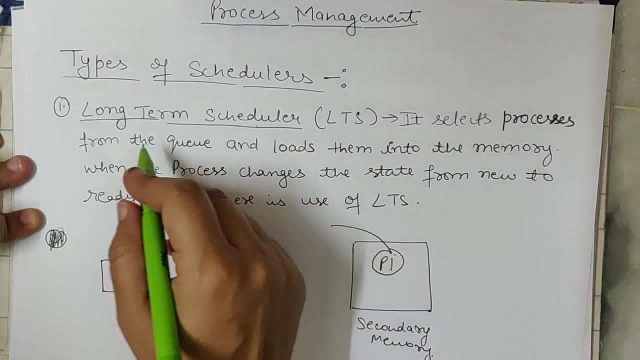 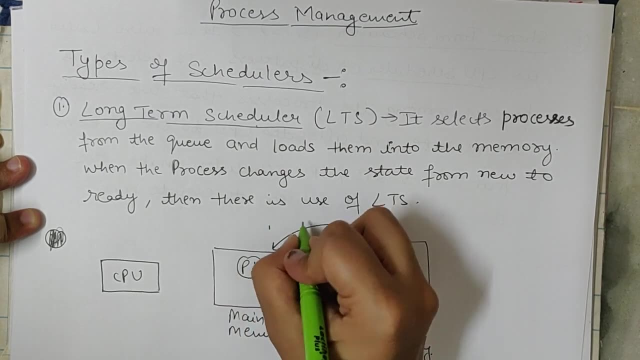 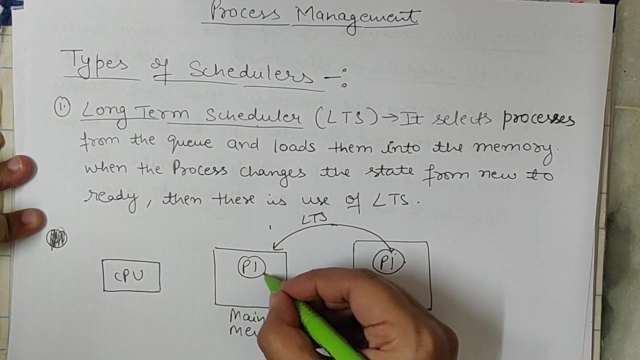 this particular program lts. what lts long term scheduler does is it will move the program p1 to the main memory. ye job hai lts ki. this is a program okay, and now this is a process, newly created process, which is ready for the execution. okay, so ye hi kaam hai lts ka. 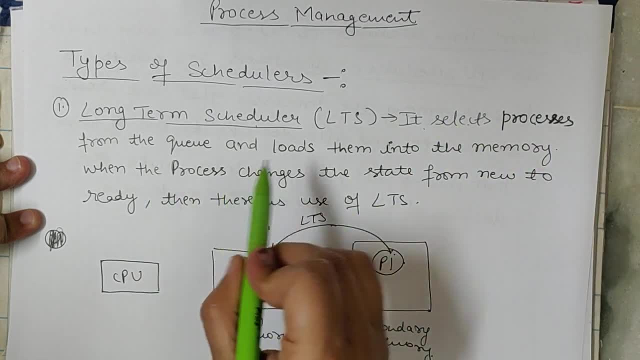 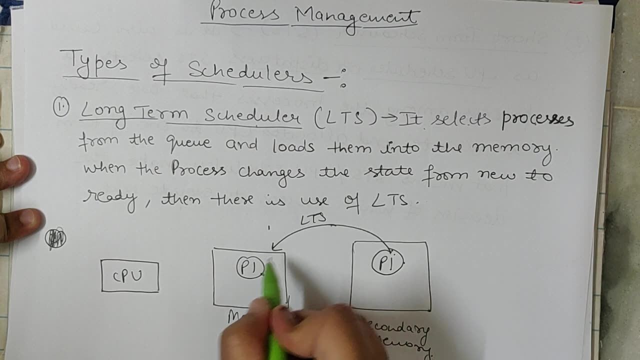 it selects the processes from the queue and loads them into the memory, main memory. when the process changes the state from the new to ready state, new means it is newly created process and now it is ready for the execution. when the process changes the state from the new to ready state, then there is a use of. 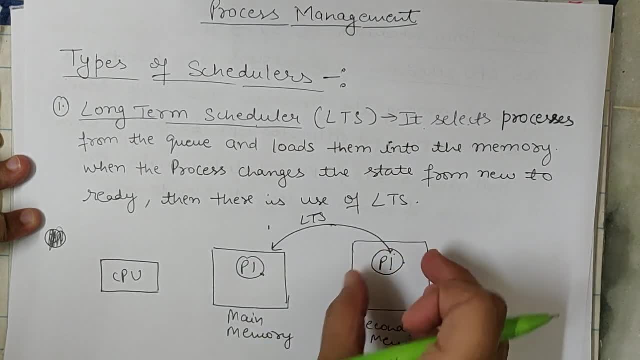 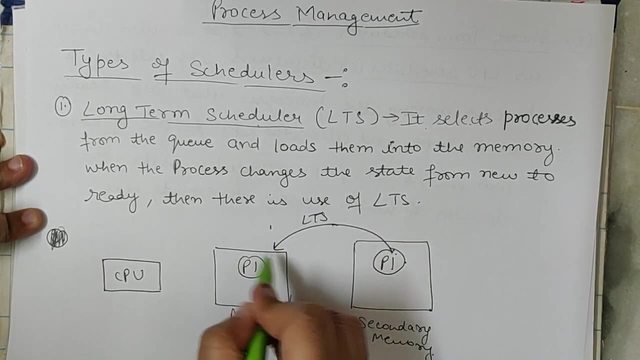 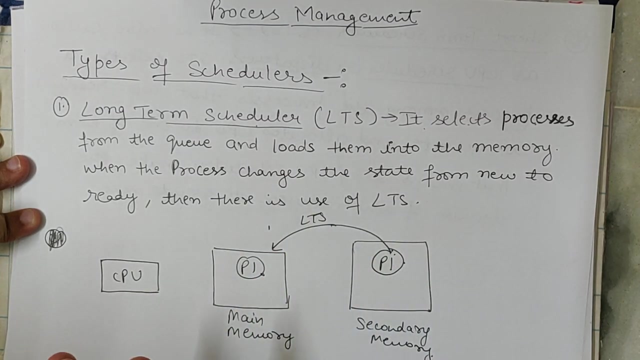 lts. so the main objective of lts is put this program from the secondary memory to the main memory and now, if this particular newly created process is ready for executiion, so there is a use of lts. so lts ki job. i hope apko clear ho kya play isku. if you know about lts ayo. 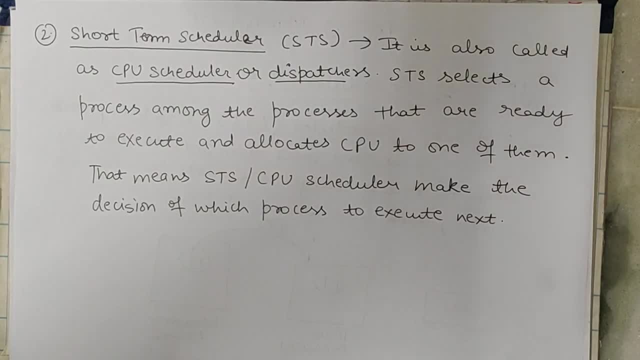 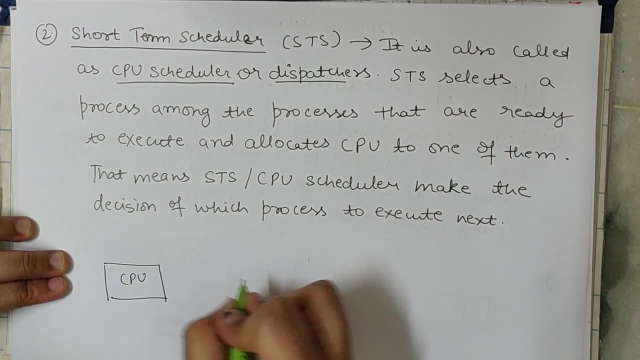 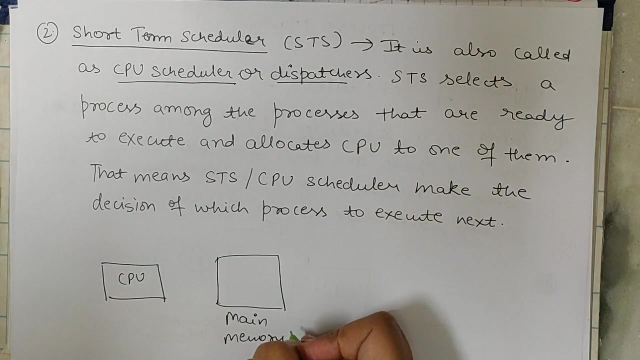 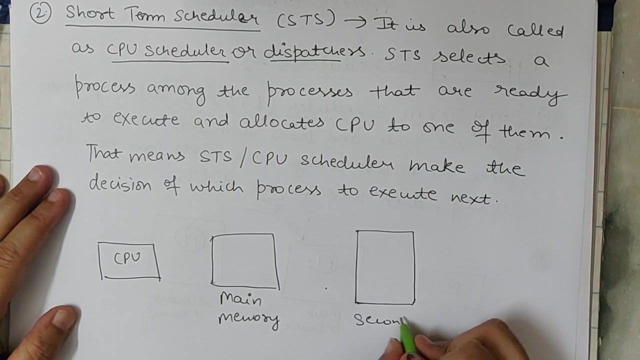 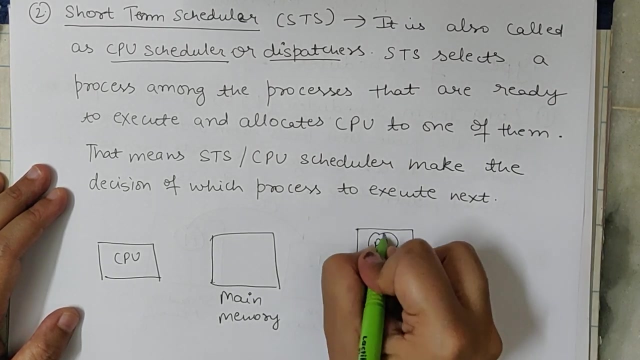 clear ho gaya hoga. lts kya karta hai. now, the second is short term scheduler. abhi hum dekta hai. isko ek example: se this is a cpu, this is main memory, main memory, this is a secondary memory, secondary memory. so this is my program p1. lts ki job kya hai? lts kya kaam, kya hai? 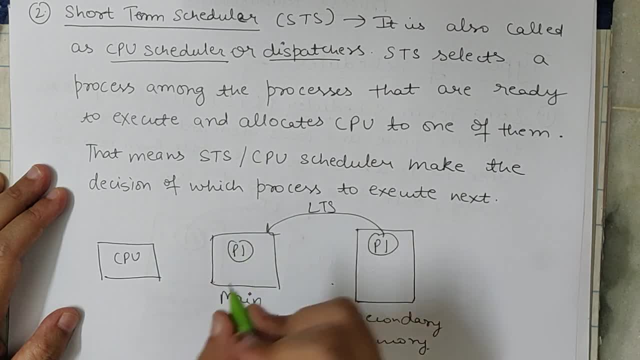 p1 ko main memory me load karna. now, say suppose i have program p2, p3 also. so lts ne p2 ko bhi move kar dia, p3 ko bhi move kar dia, all are in. all these three processes are now present in the main memory. so this is my program p1. lts ki job kya hai, lts, kya kaam kya. 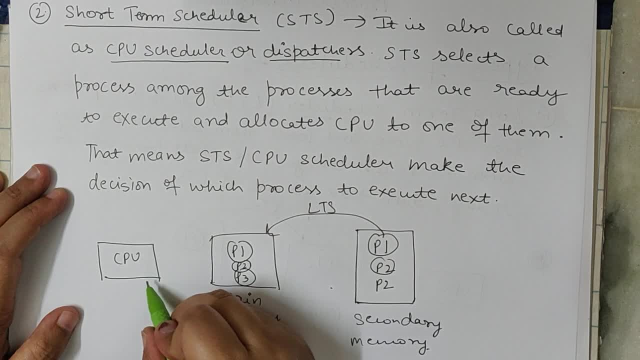 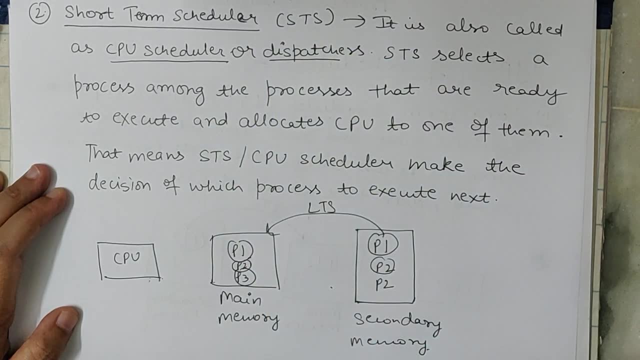 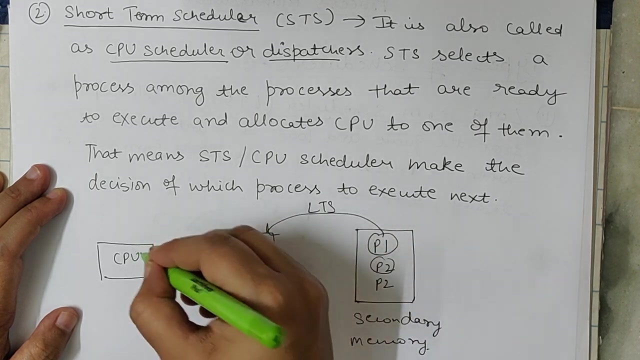 main memory and they are ready for execution. but we have only one cpu at a time. only one process will get a chance to access the cpu. so what the job of sts is? it selects one of these processes from the main memory and allocate the cpu to one process. ok, so yeh decide, karega. 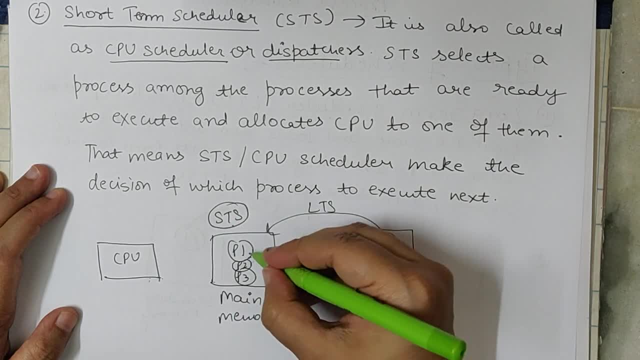 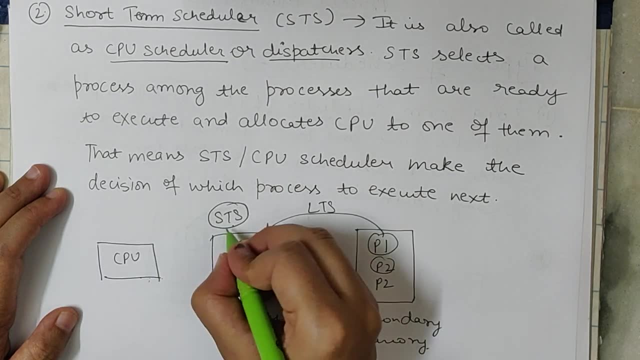 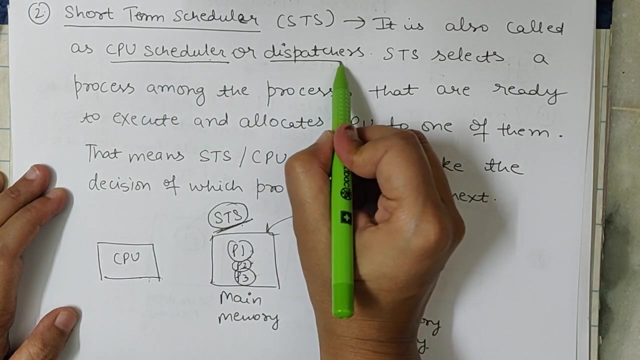 kaun sts short term scheduler ki responsibility hai: p1, p2 aur p3 in tino mese kisko cpu dena hai, pehle kisko cpu dena hai. yeh decide korn karega short term scheduler. and this short term scheduler is also known as cpu scheduler aur dispatcher. okk yeah, though, say suppose. 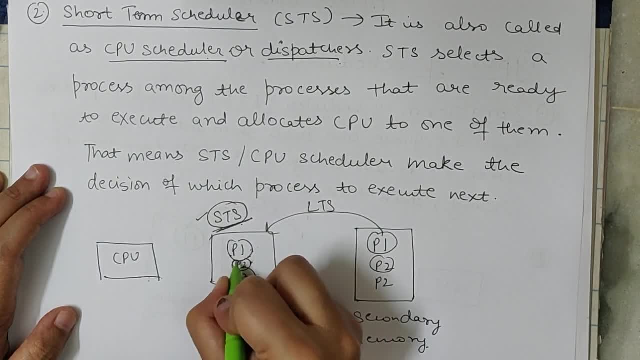 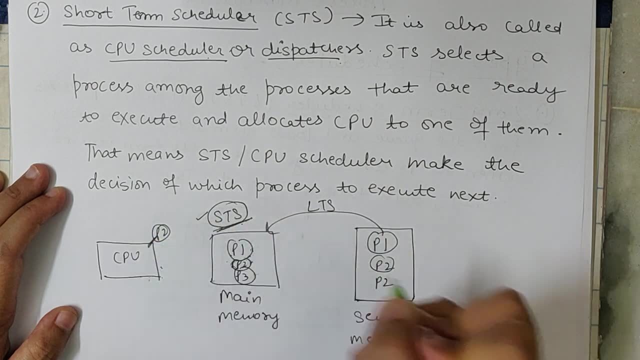 sts ne decide kiya, i will assign the p2 process, i will select p2 process for the allocation of cpu. toh p2 process ko pehle cpu melega, toh yeh job viska hai. sts ka long term scheduler ki job kya hai. load karna hai secondary memory se main memory me saare processes ko skills. 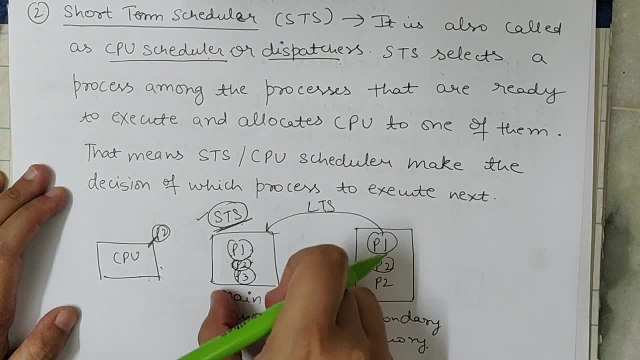 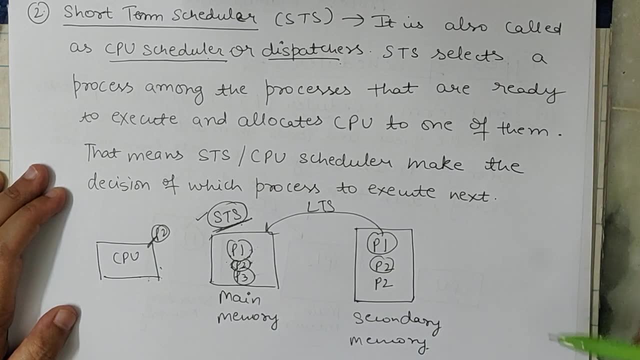 necessary nLES فirar. so let's dig into. give one example first. let us say: if this is the, What is the responsibility of STS, Who should be given the CPU first? That is the responsibility of STS. So you can take a screenshot. 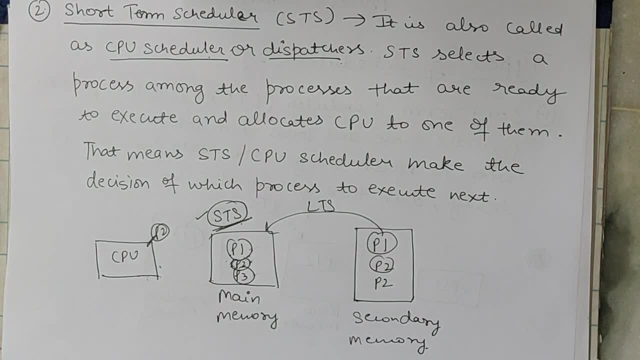 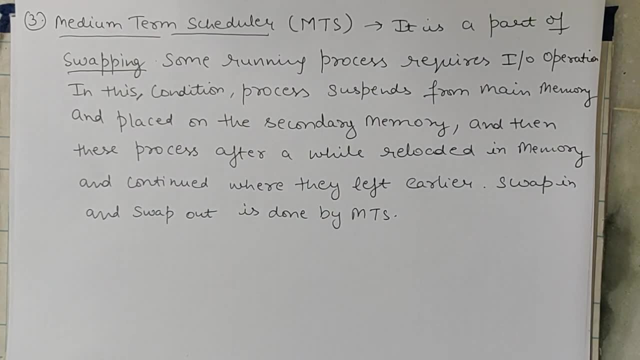 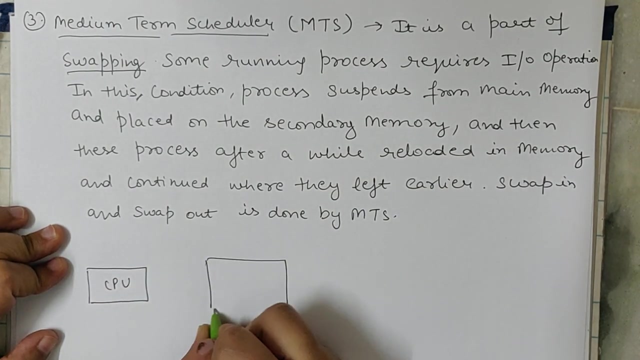 This is the full explanation of short term scheduler. If you want, you can take a screenshot also. The third one is medium term scheduler, And this is also known as swapping. So let's explain this with an example. This is a CPU, This is a main memory And this is secondary memory. 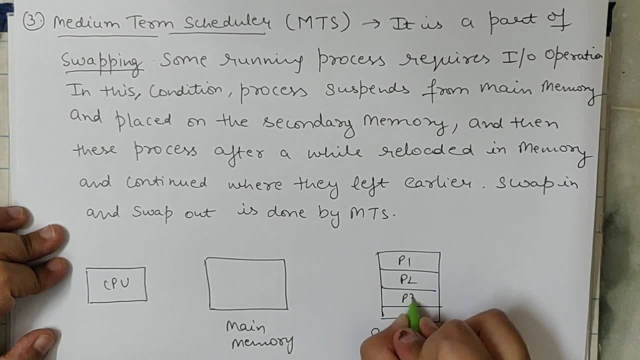 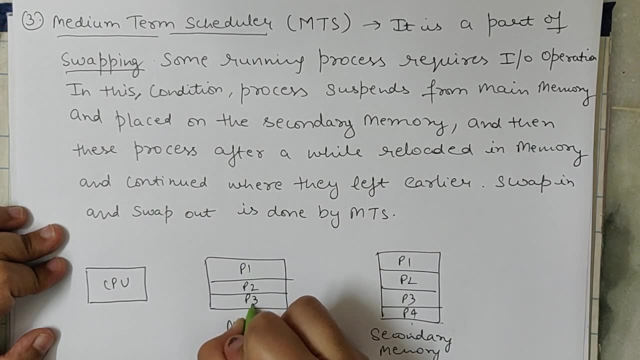 So we have P1, P2, P3, P4 and so on inside the secondary memory And we want to execute P1,, P2, P3. So it will be resigned in the main memory, But at a time only one process will get a CPU. 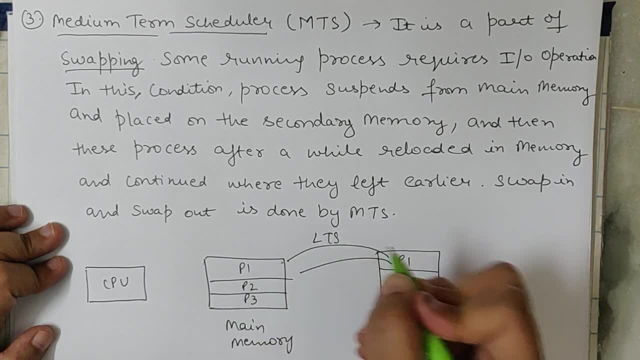 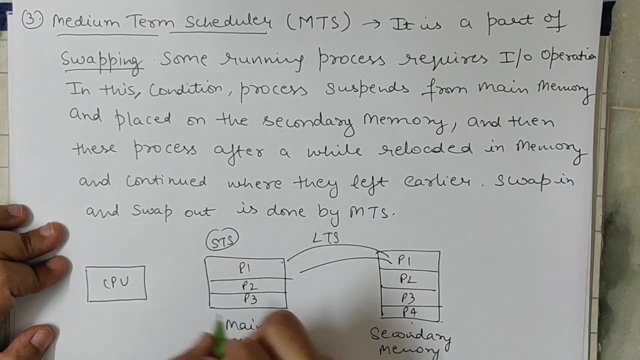 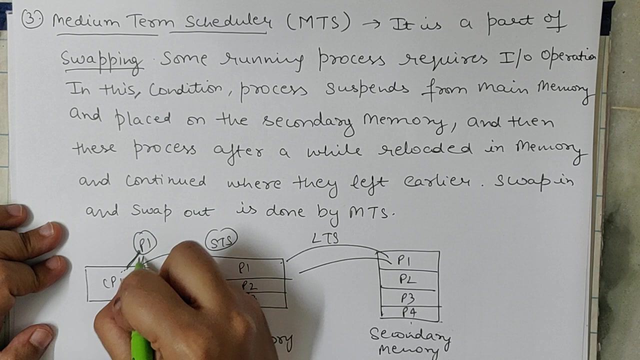 This process is done by LTS From the secondary memory to main memory, And who decides who will get the CPU? STS decides P1 will get the CPU first. So P1 is accessing the CPU And in between the execution, P1 process wants to access a particular resource.